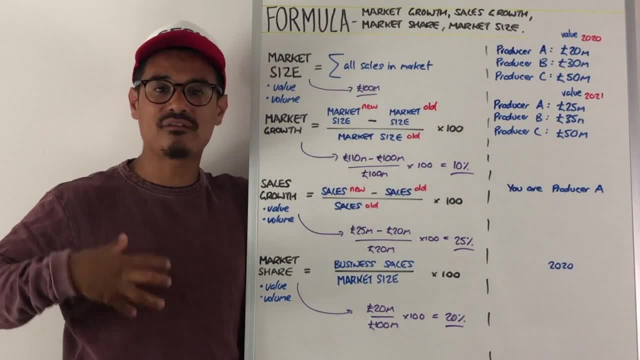 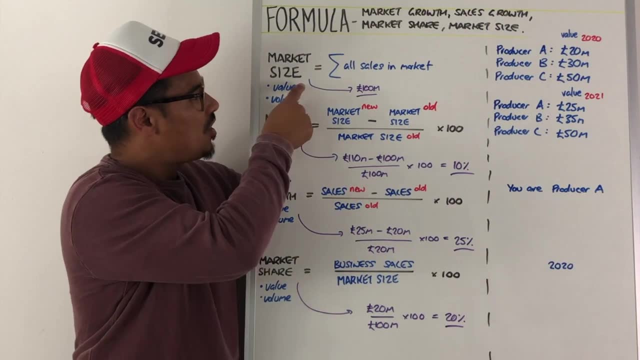 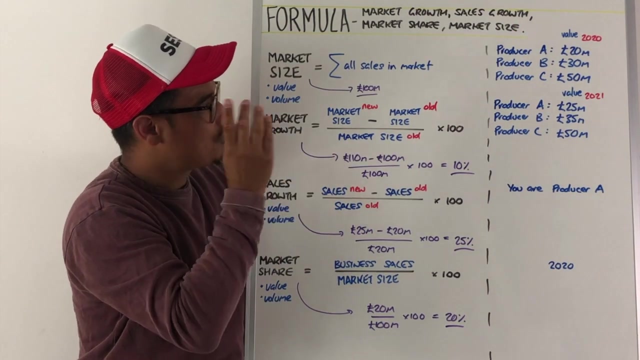 pounds. If it's volume, it's in the amount of units, so the amount of things sold. So formula for market size is the sum of all the sales in the market by either value or volume. The question will tell you that. Let's look at some data here. So we're going to get the market size based on value: Value in. 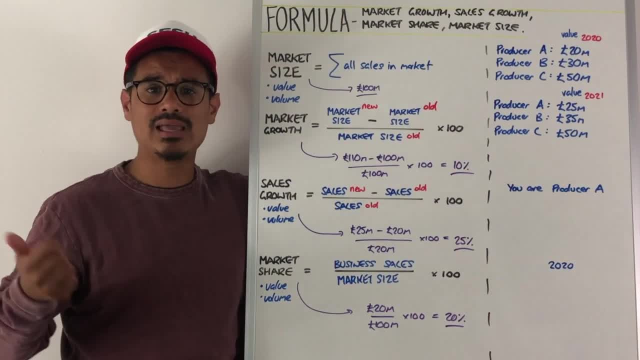 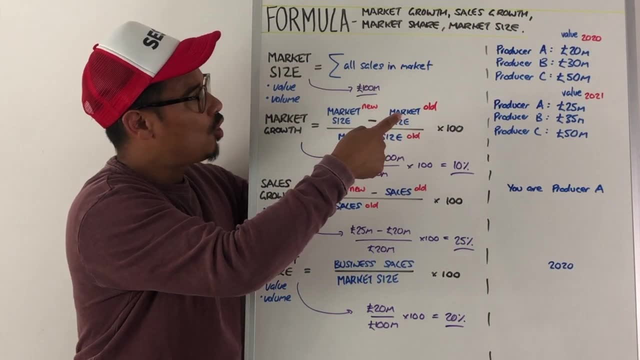 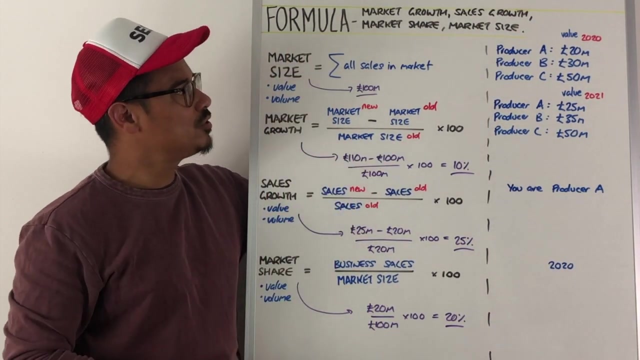 2020.. There are three producers, three businesses in a market- A, B and C- and they have respectively 20 million, 30 million and 50 million pounds worth of sales in terms of value. of course, The market size is just add them all up. add all the producers up and the producers comes to. 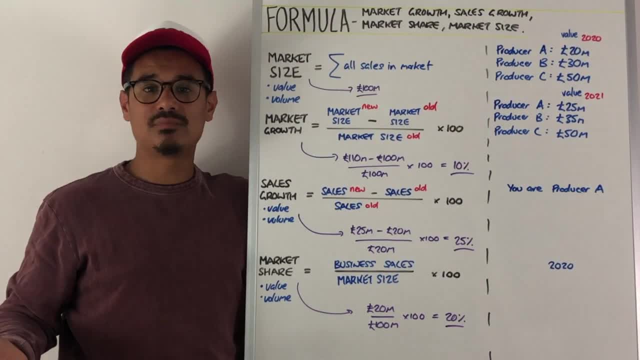 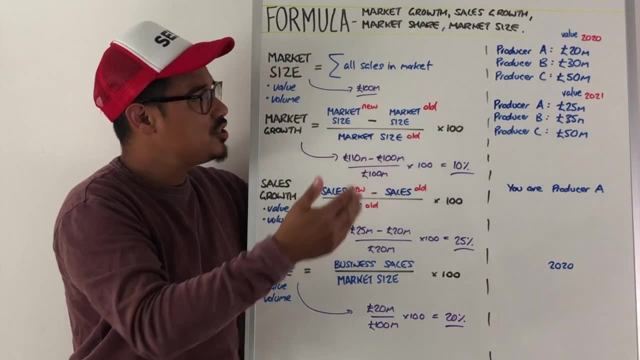 a total of 100 million. 20 plus 30 is 50, 100 million pounds. Easy peasy. The next one is market growth. Market growth. the formula is: market size in the new year, in the latest year, in the current year that the question is asking for you, minus the market size in the old year. 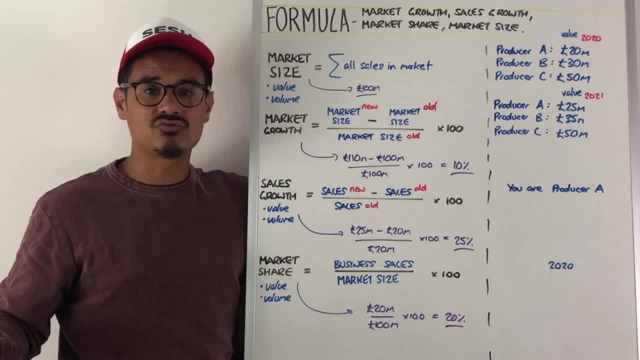 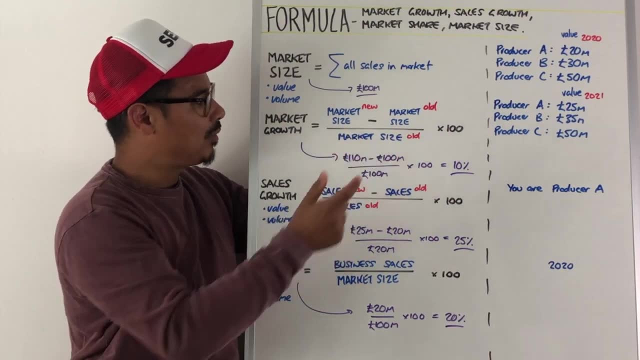 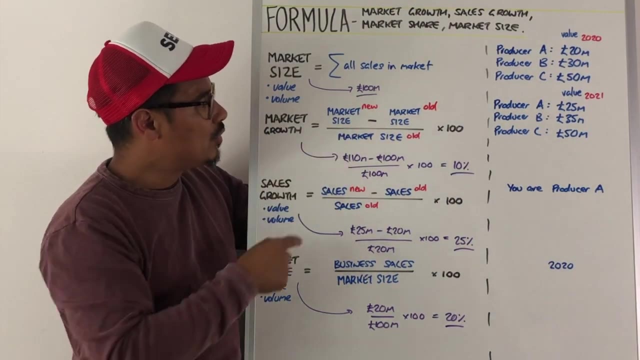 All divided by market size in the old year times by 100.. You're just thinking percentage changes here: New, new minus old, divided by old times by 100. So we apply some data to that. If the question is, what is the market growth between 2020 and 2021, then we need to get the market. 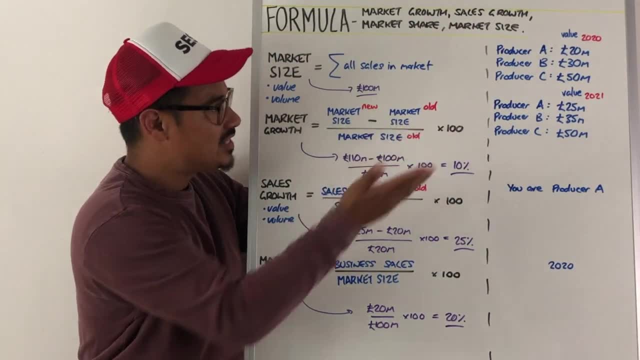 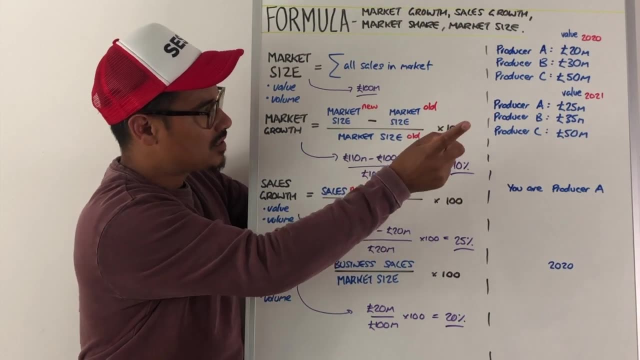 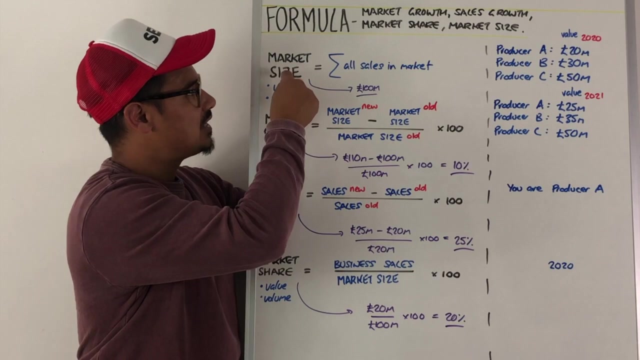 size in the new year. The new year, the latest year, is clearly 2021.. That's the most up to date year And the market size in that year is by adding up all those producers. So 25 plus 35 plus 50 is 110.. 110 million minus the market size in the old year, which we calculated in the 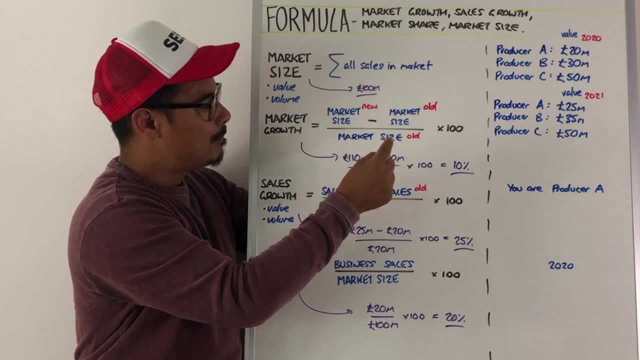 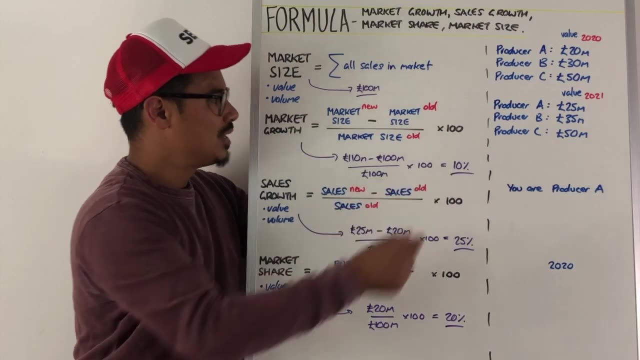 previous bit, 2020 is 100 million, 110 minus 100, divided by 100 million for all of them, times by 100 to put it in a percentage, And that comes to 10 percent. So the market size in the new year is: 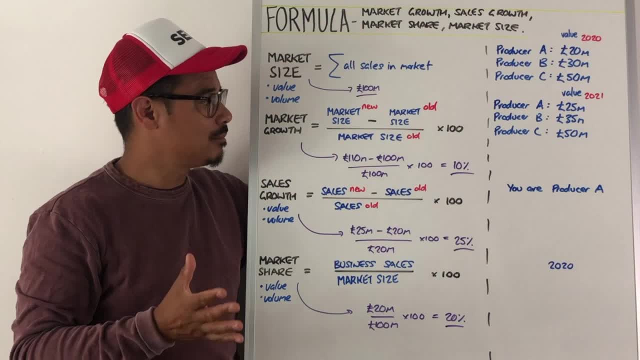 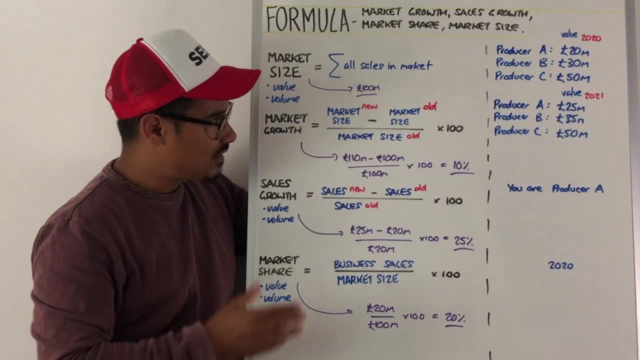 by 10 percent. The market growth was an increase in 10 percent by 10 percent. The next one is sales growth. Sales growth: always check if it's by value or by volume. Here we're sticking with value, with our data up there, And the formula is going to be: your sales in the new year, the latest year. 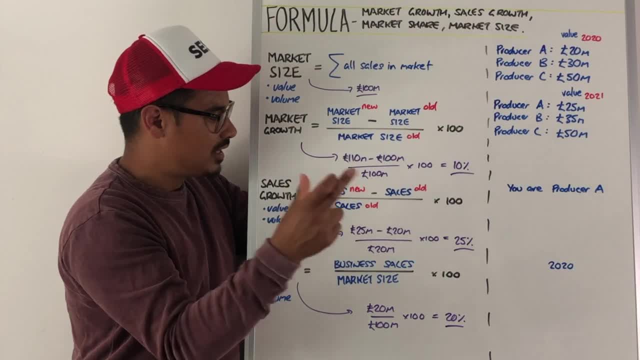 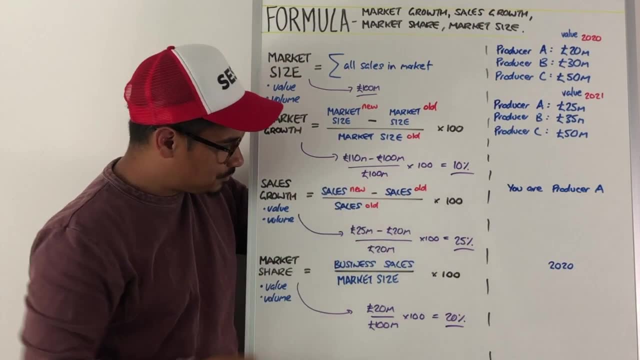 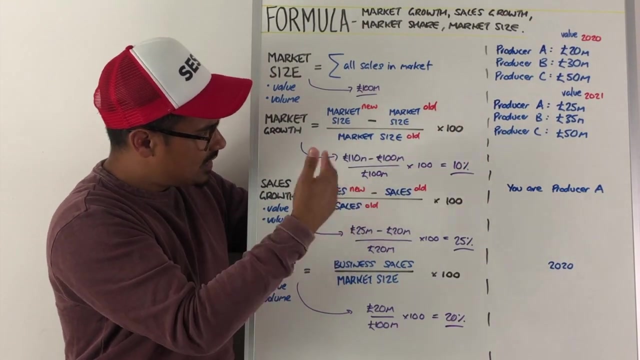 the current year minus the sales in the old year, all divided by the sales in the old year times by 100.. So if we do that and say that we are producer A and we're looking for what the sales growth was in 2020 and 2021, we get the most up to date year 2021.. And that was if we're producer A.